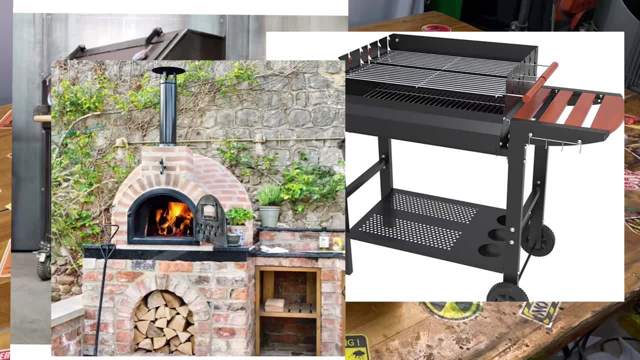 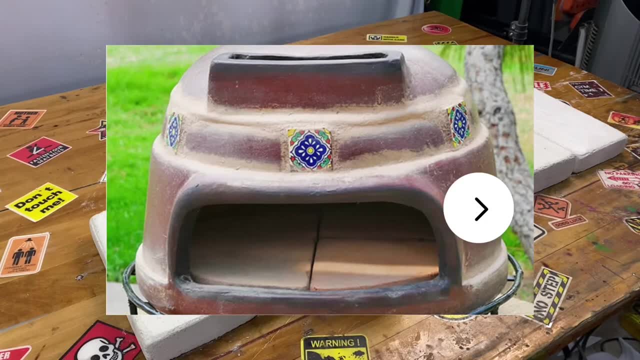 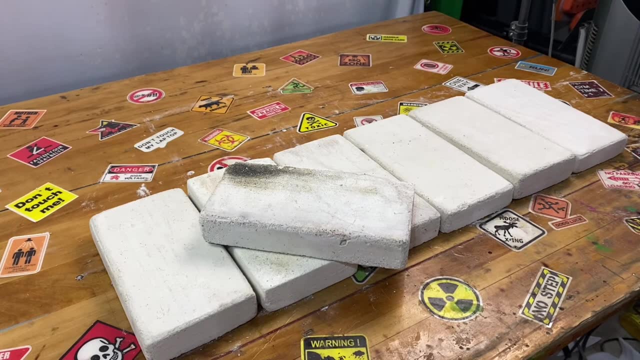 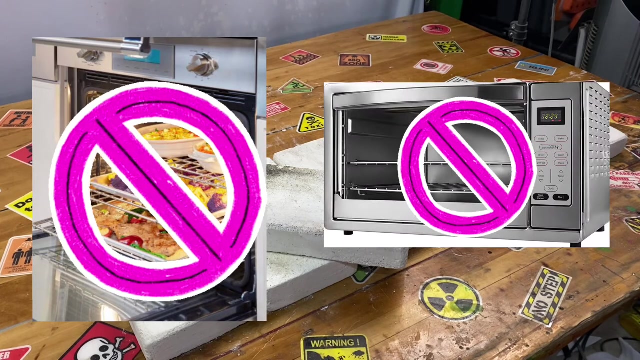 pizza ovens, propane forges, electrical furnaces, maybe even a tile pizza oven. It's pretty self-explanatory what not to use them for. I mean, I probably wouldn't use them for my conventional kitchen oven or my convection ovens or anything like that. I mean. 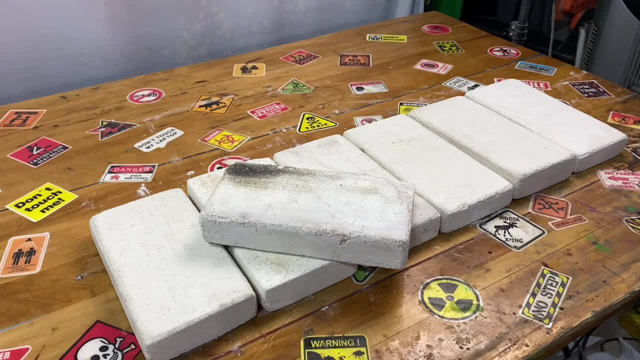 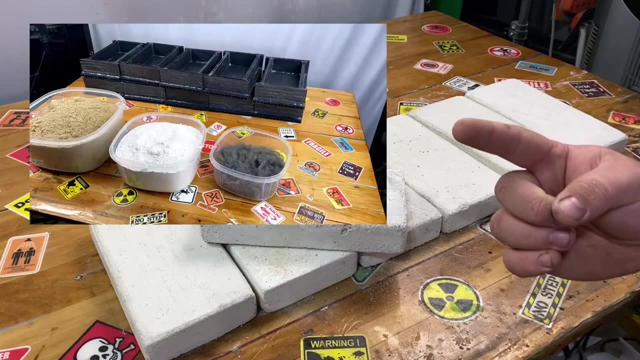 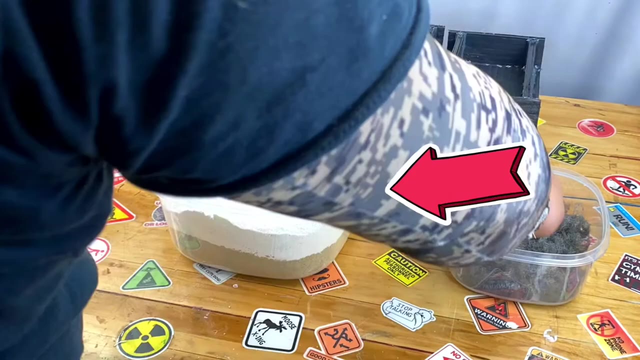 it's pretty self-explanatory. But besides that, as far as the mixture goes in my first video, if I slowed down this clip a little bit, you'll see that I pretty much did about 50 to 50.. As far as the steel wool goes, you can add: 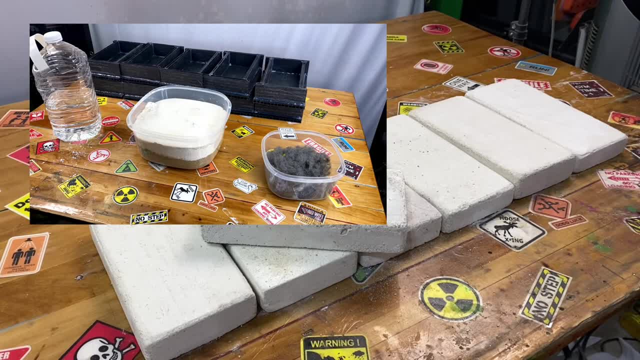 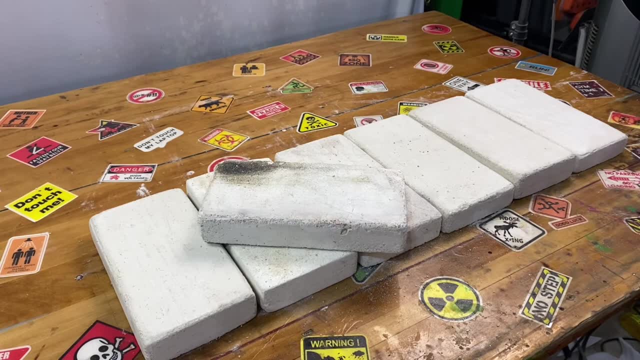 as much as you want, or you don't have to add it at all. It's completely up to you. I can't stress that enough. This is your world. You can do whatever you dream of. Now I can't tell you how. 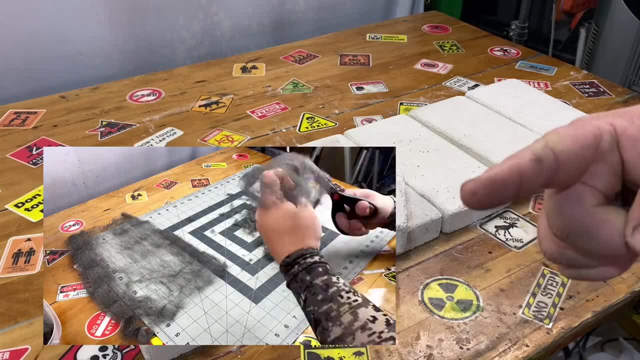 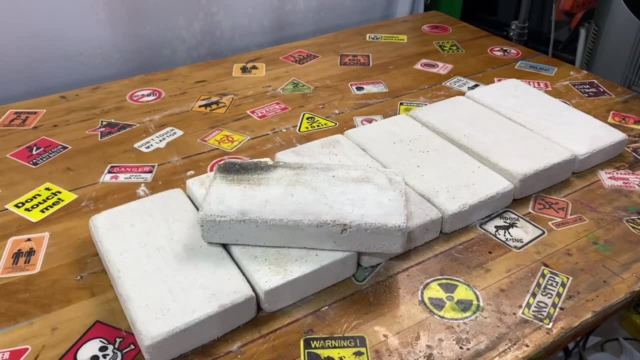 it's going to turn out. But once again, if we look at this section of the video, I mean, if I had to guess, it's probably a small strip of that in each and every single one of these, solely based on how much. 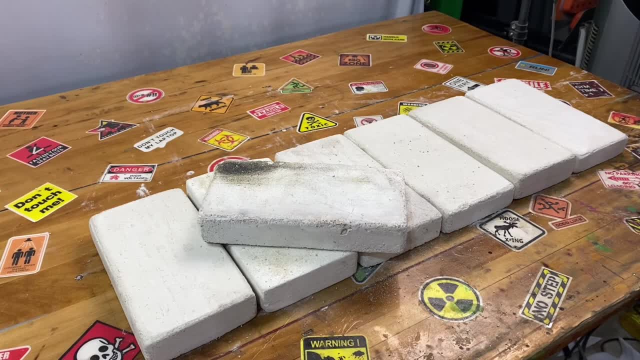 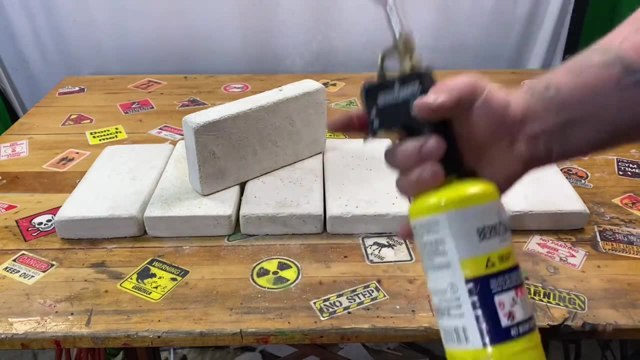 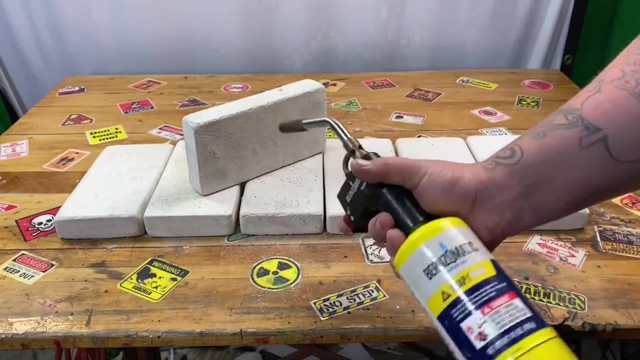 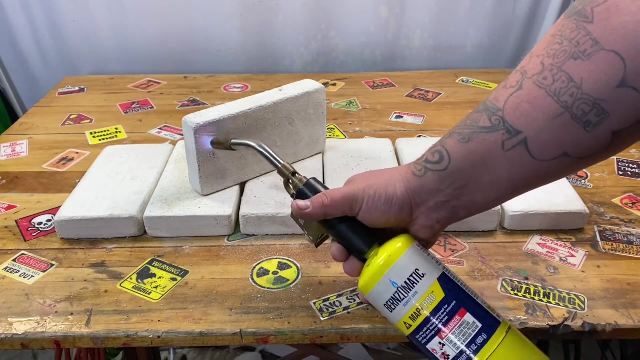 I threw in the container while I was mixing it. So some might have more, some might have less. So originally I only planned on using the MatPro handheld torch to simply get something up to the most, maybe 700 degrees. If we set an example right here and I heat up this corner, the surface of it would get, you know, a little red. sure, not too much. 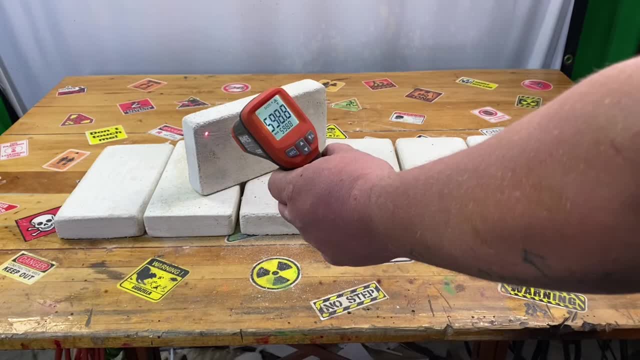 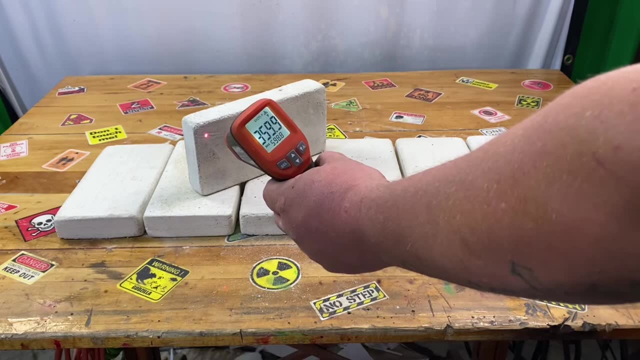 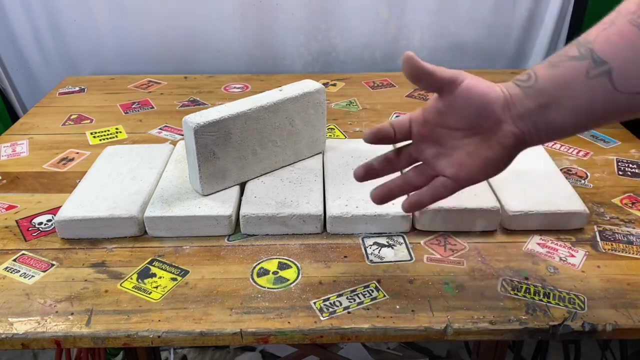 We'll see how hot that is. That's about 500.. And see how quickly it lowers down. That's how much the heat is escaping from this thing. That's really easy to help melt stuff that is lower temperatures, like gallium or copper. 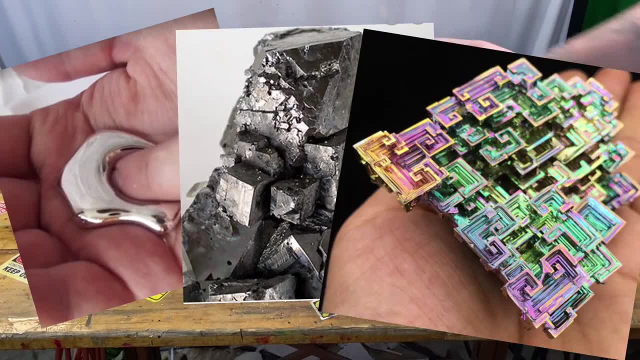 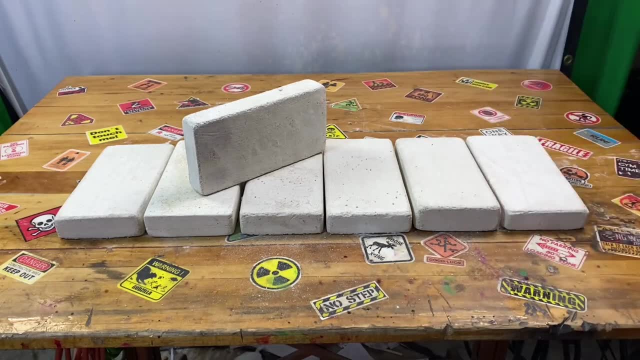 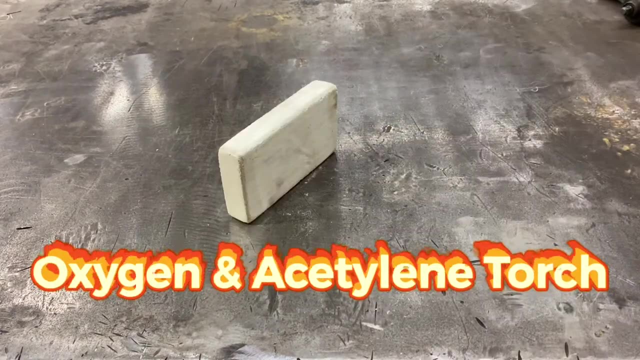 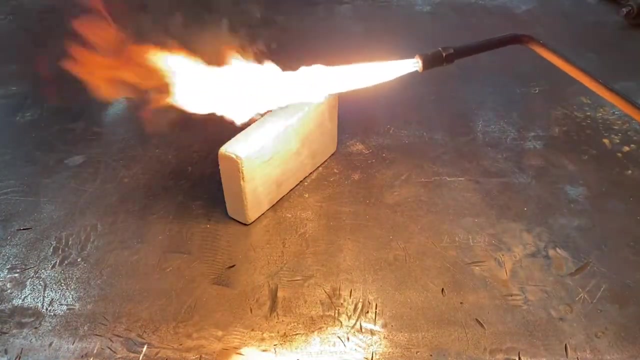 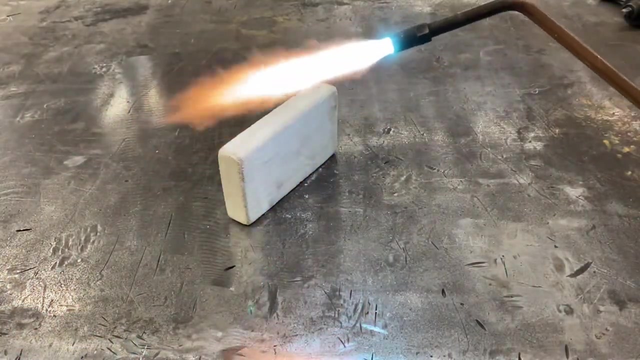 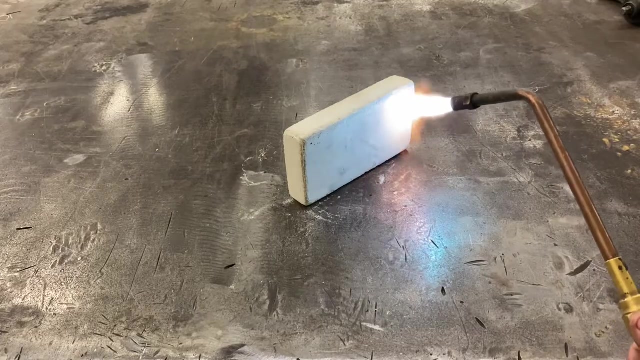 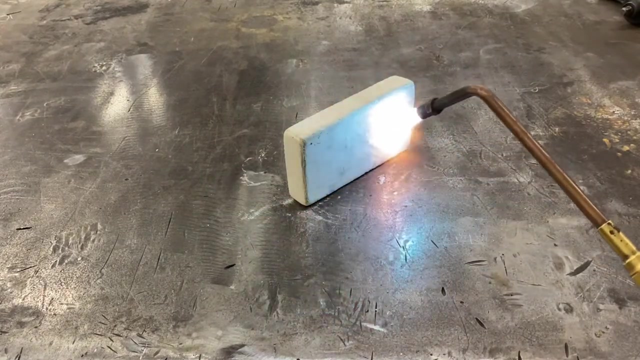 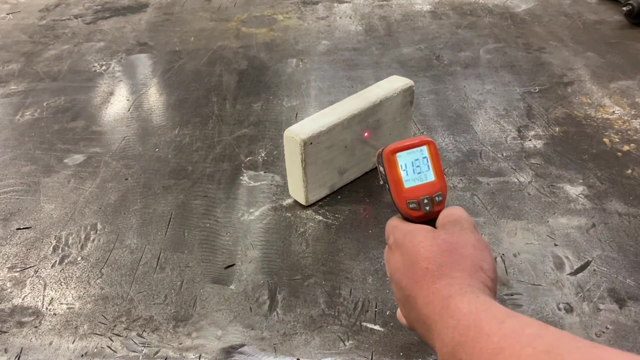 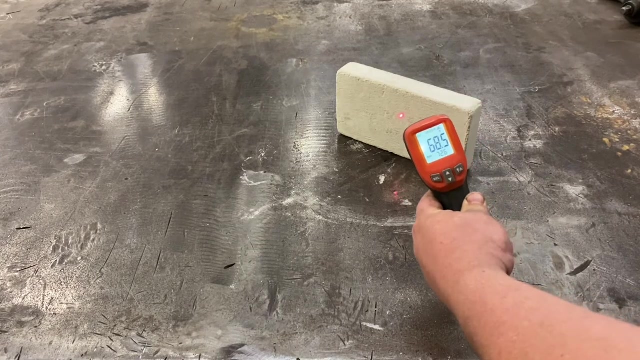 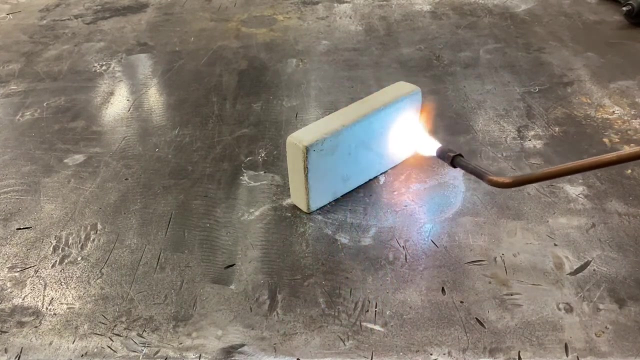 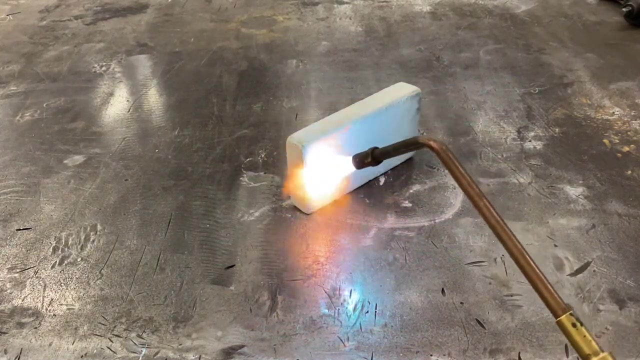 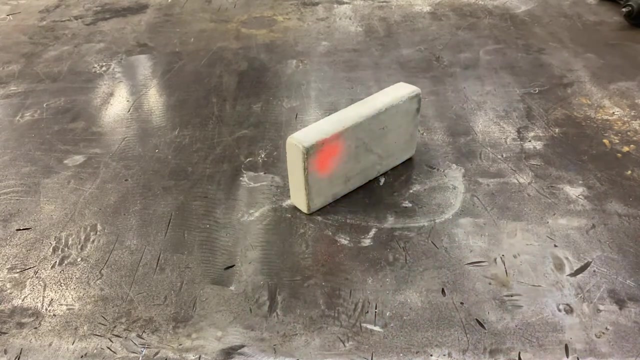 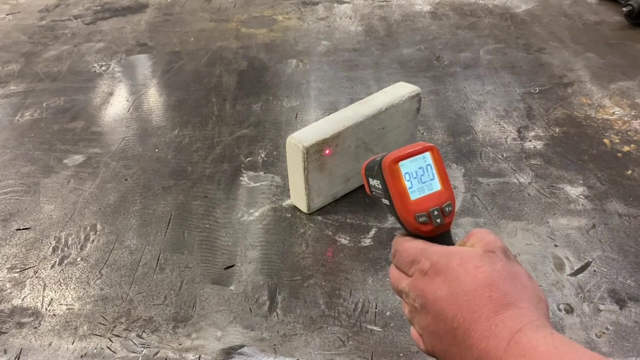 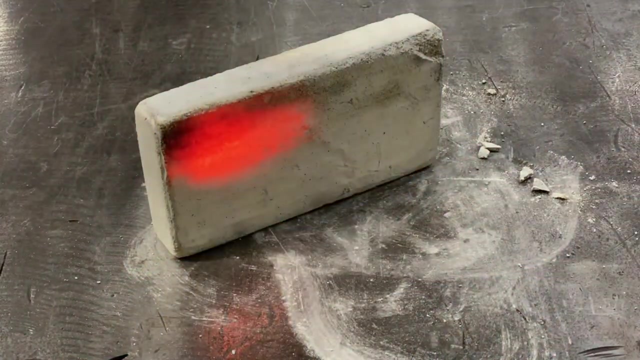 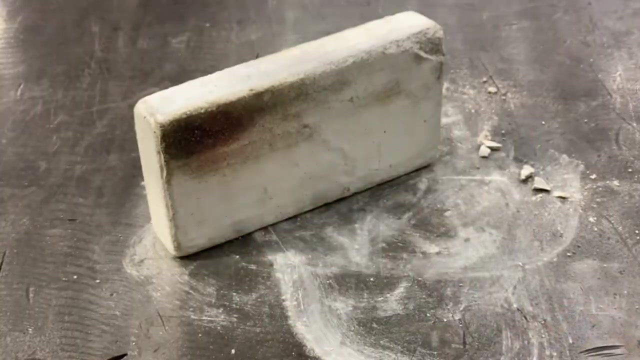 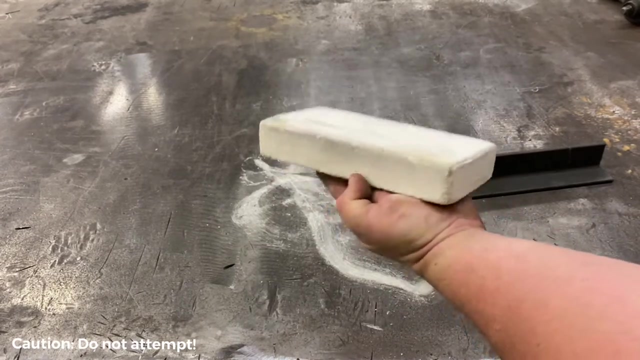 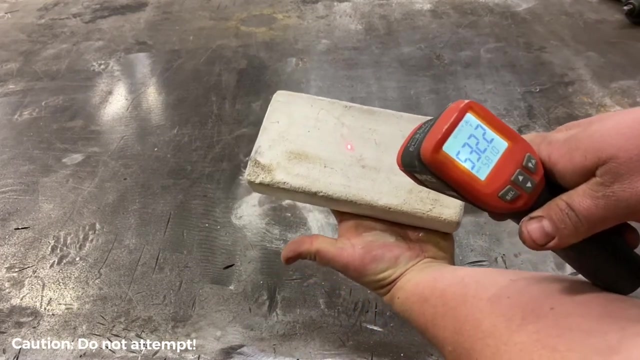 Lead or bismuth, something to just have fun melting metal down with. But since you guys want more of a higher heat test, let's take it up a notch. Okay, Thank you for watching. Thank you for watching. 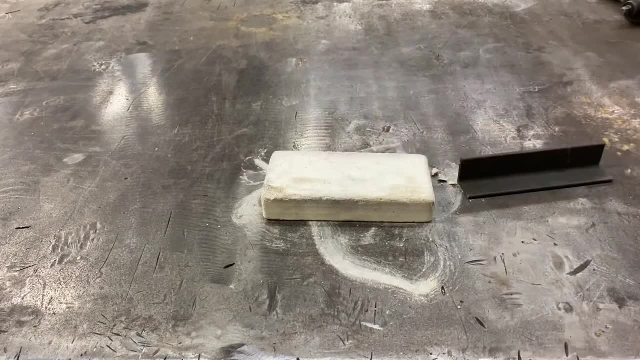 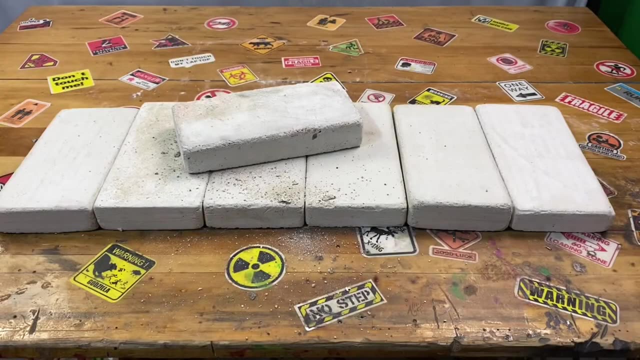 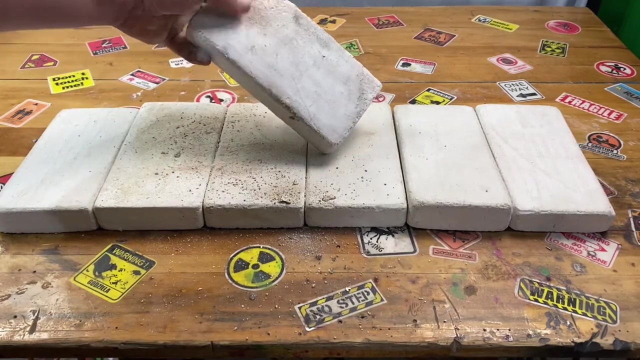 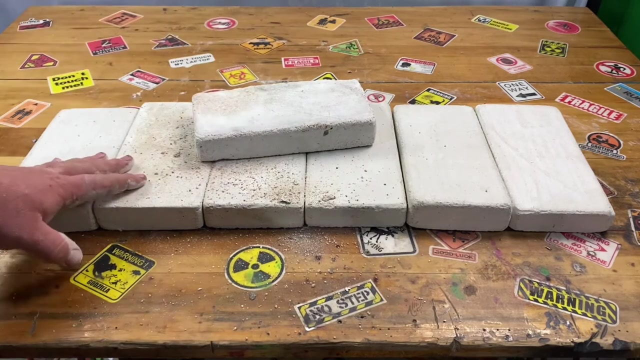 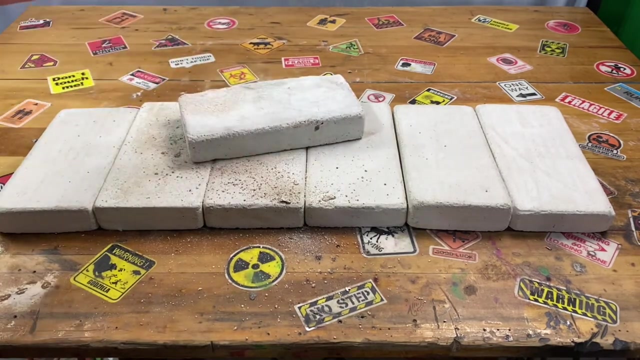 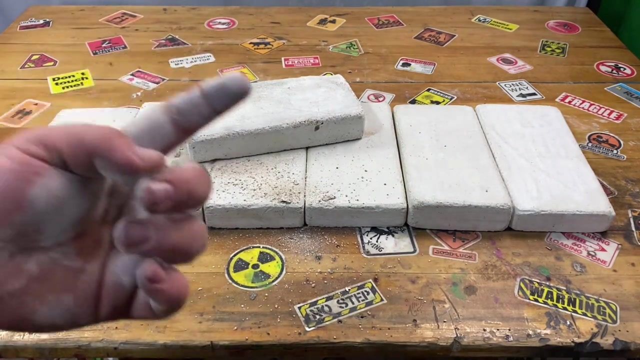 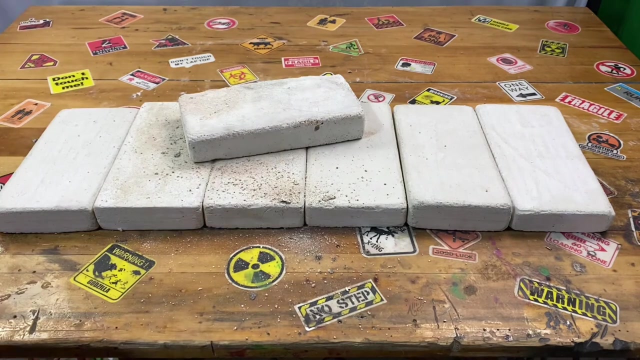 Thank you for watching. So if you guys want to see more detailed experiments or testing, check out the King of Random in the top right corner. He has made a metal melting foundry that actually puts this stuff to the test a little bit more. 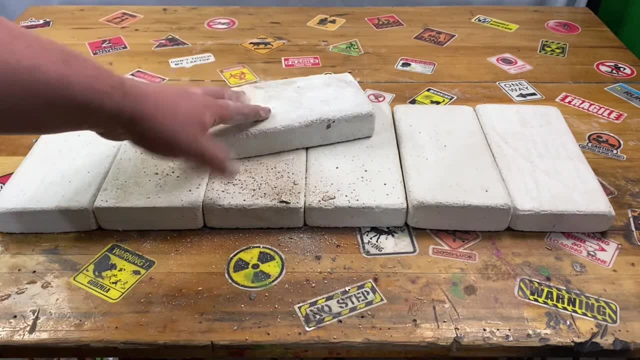 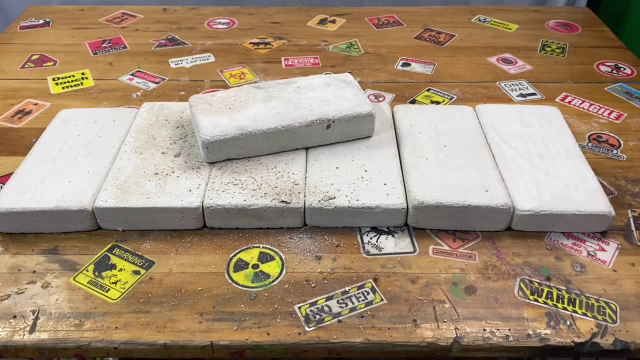 And we both have pretty similar mixes. So I thought it was a pretty cool video to check out And once again, I'll leave that in the top right corner for you guys to see. So I'm done with the test myself. 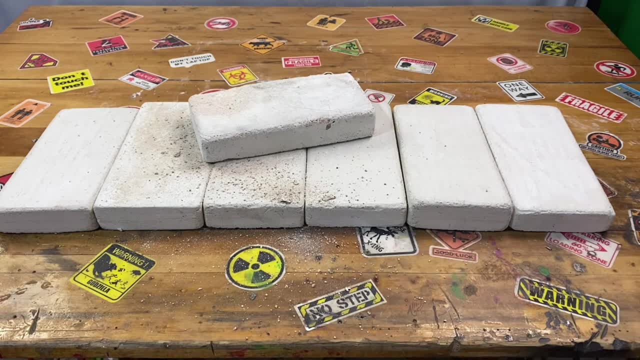 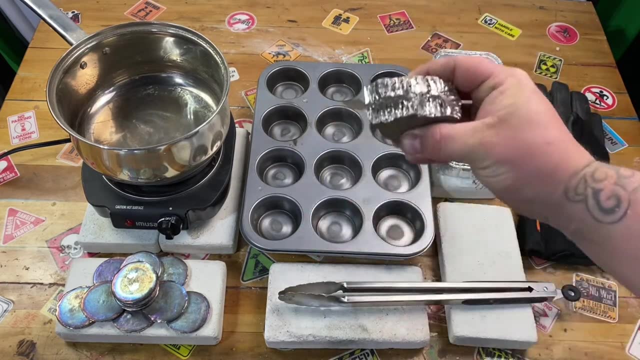 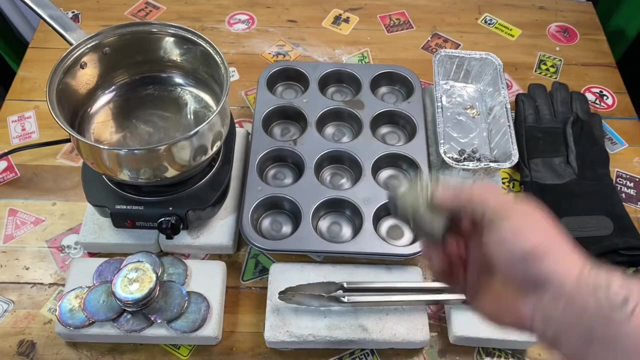 So I say let's have some fun and melt some metal down. Alright, So pretty simple setup. We will be melting down some bismuth, which is a geometrical metal. So once this gets to a certain temperature and it gets cooled down, it will actually create geometrical crystals. 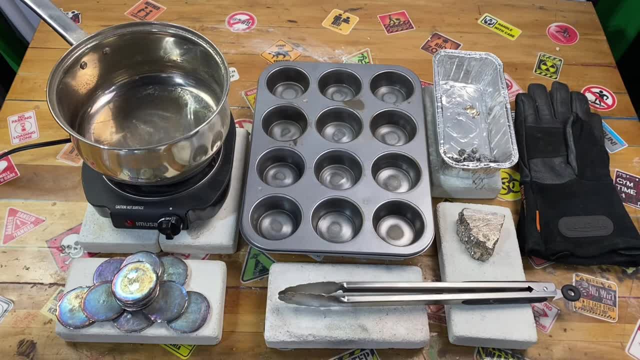 And the stuff looks amazing. So it melts around 520 to about 520.. So we're going to let it cool down to about 550 degrees in order to get those crystals to shape. We want to get it hot and then let it cool itself down. 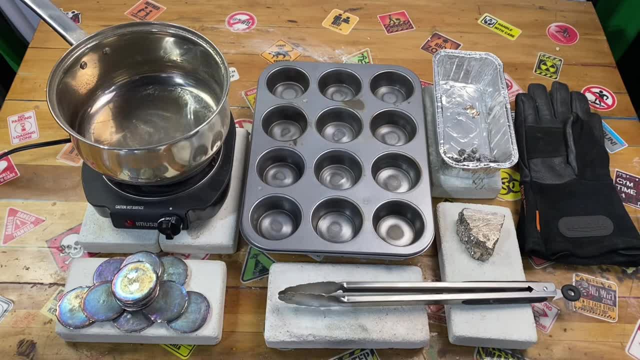 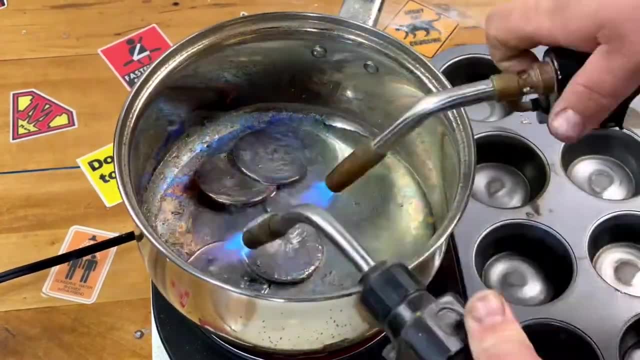 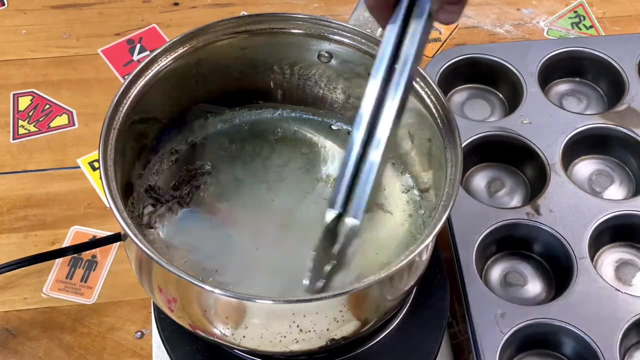 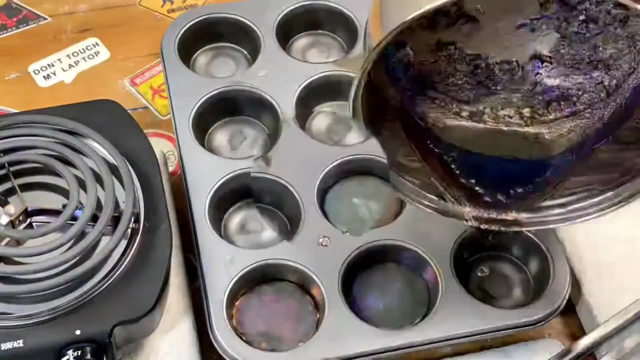 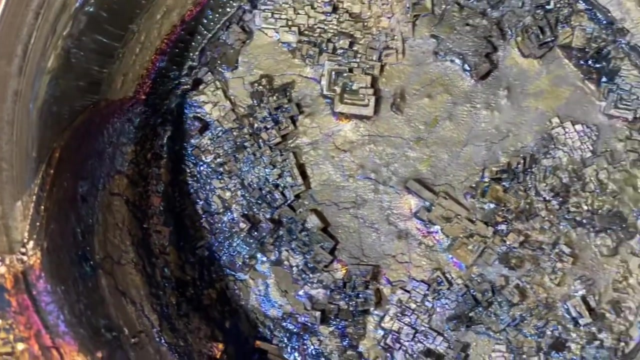 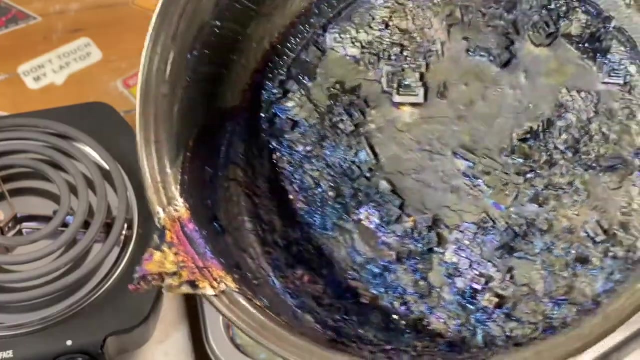 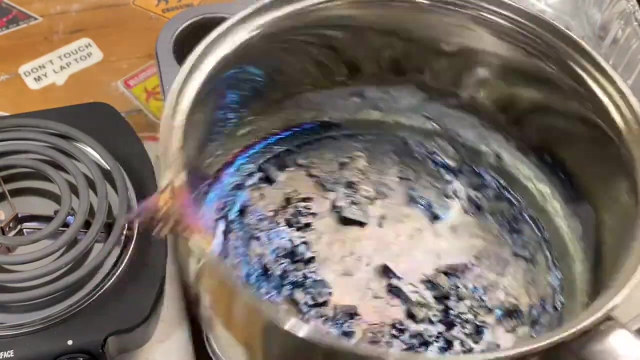 And let's see if we can't reheat it up and let those crystals rise to the surface. Alright, So let's get the improved out. it's like Good, there you are. I'm not sure I can do that.